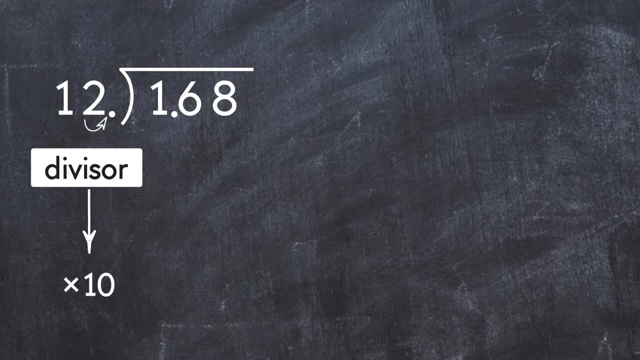 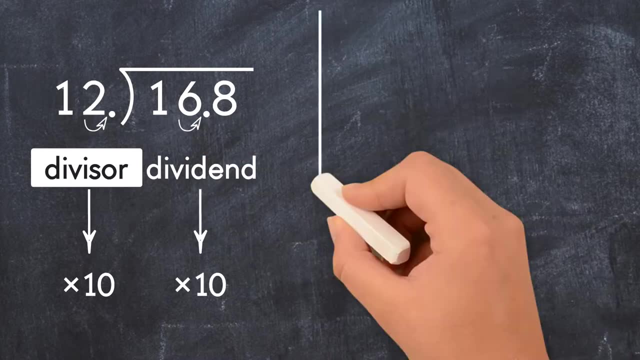 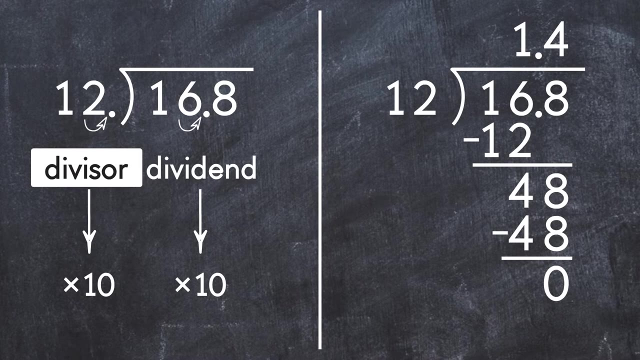 We multiply by 10.. Remember, we also have to multiply the dividend by the same number, 10.. Now we have 16.8 divided by 1.2.. We solve by long division and we get 1.4.. So 1.68 divided by 1.2 equals 1.4.. 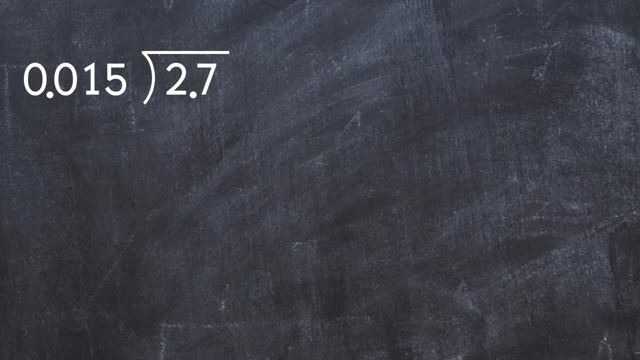 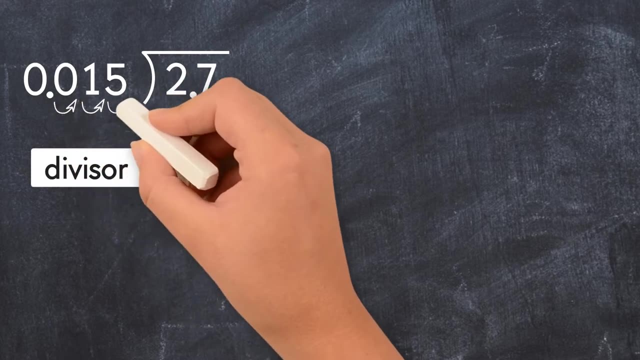 Let's do another one: 2.7 divided by 0.015.. To get a whole number in the divisor, we need to move the decimal point three places to the right. We do this by multiplying by 1000.. We also have to multiply the dividend by the same number, 10.. 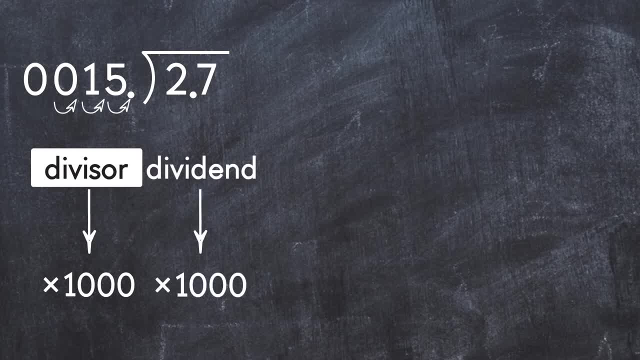 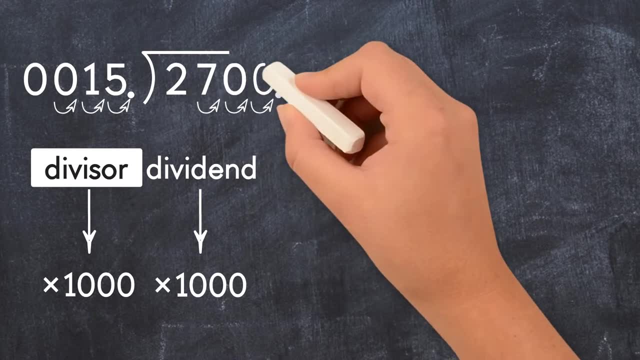 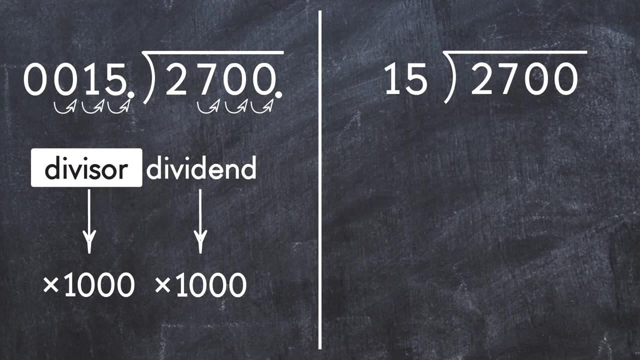 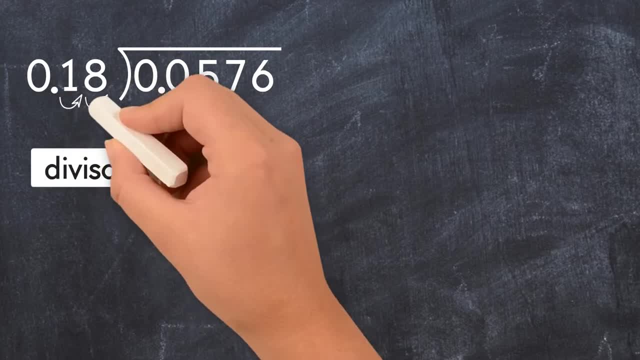 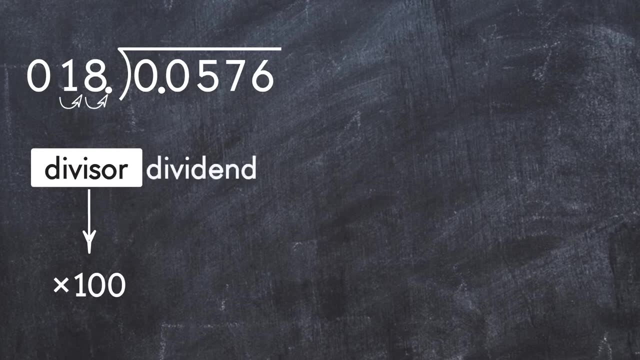 Let's do another example: 0.0576 divided by 0.015 equals 180.. To turn the divisor into a whole number, we need to move the decimal point two places to the right. We do this by multiplying by 100.. We also have to multiply the dividend by 100. 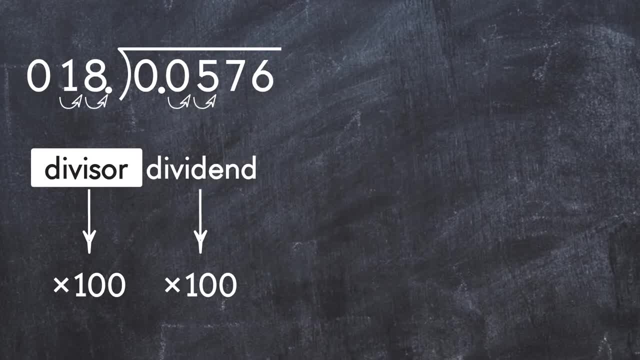 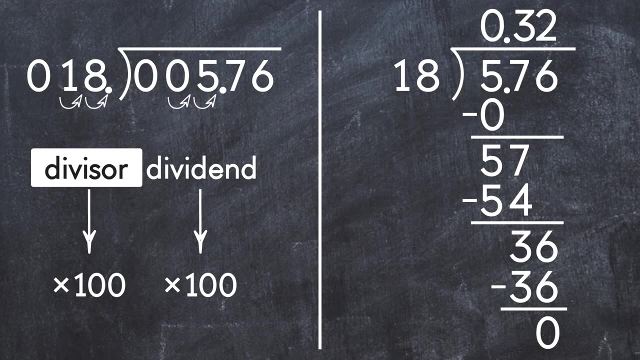